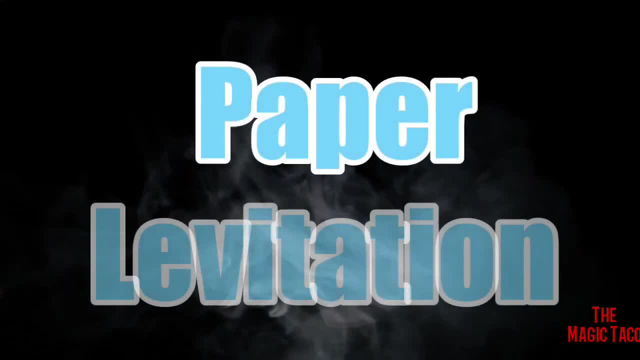 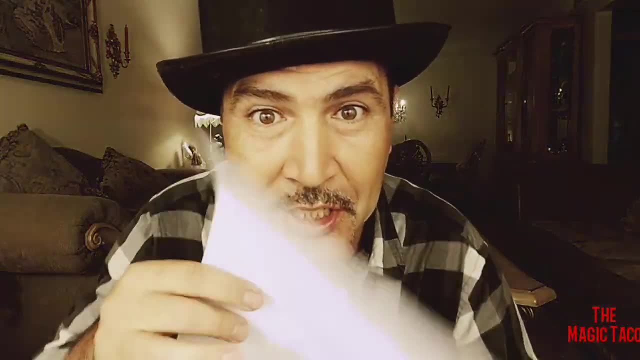 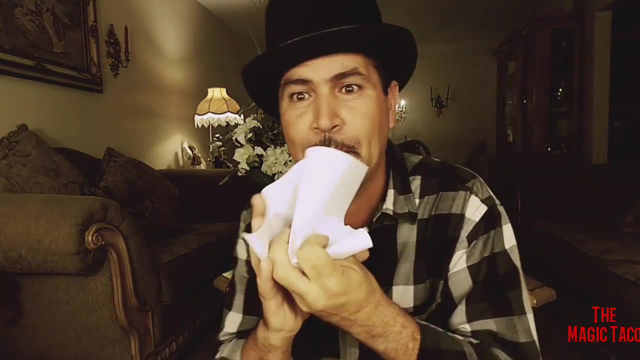 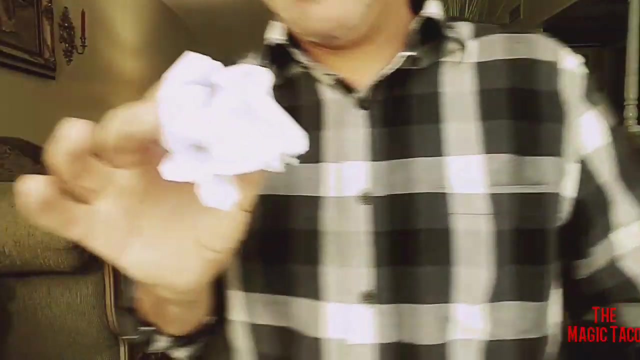 Well, boys and girls, for the next treat you need a piece of paper, Check this out. all you got to do is just grab that paper and wrap it up into a little ball like so, Check this out. and all you do is just grab that piece of paper, place it. 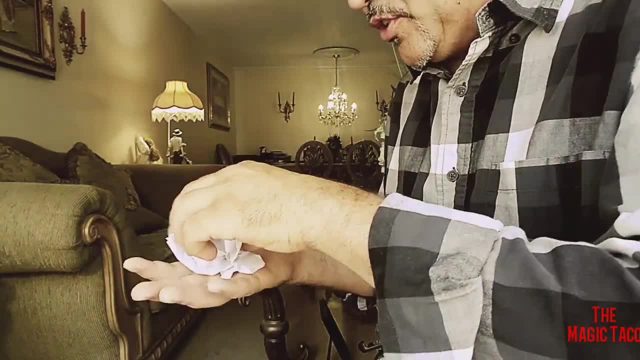 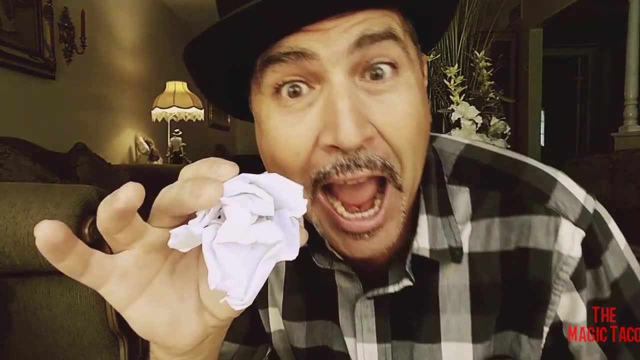 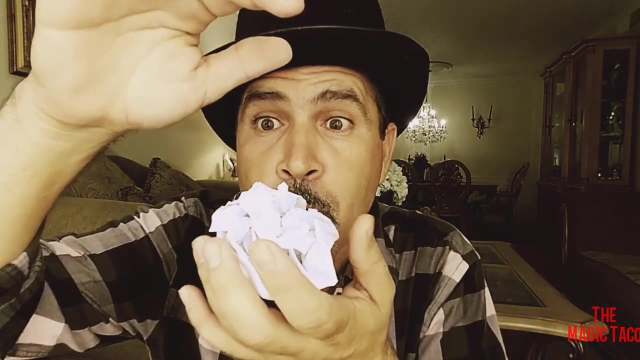 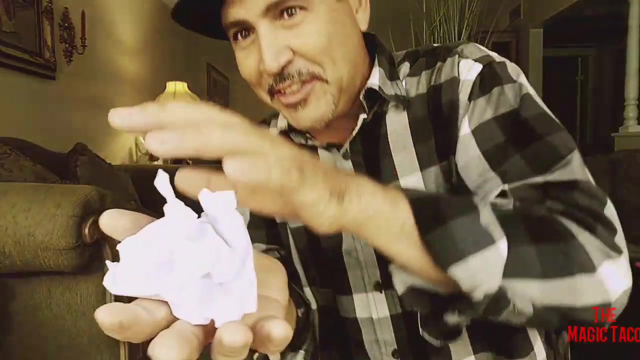 right there in your hand, like so, okay, and all you do is just concentrate on the paper. Put something in the air and you catch it. You can even grab it like so, Place it right on your hand and blow on it Here. I'll do it one more time, check it out. here you go. All you do is just concentrate and it. 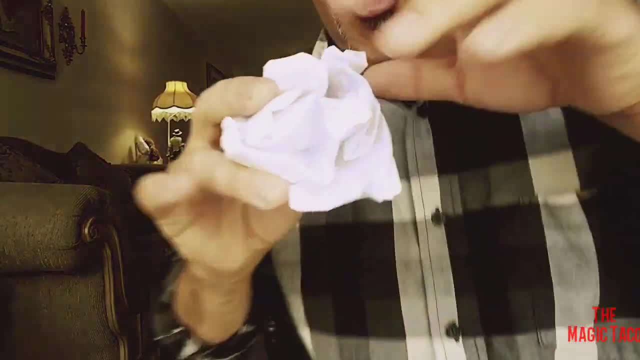 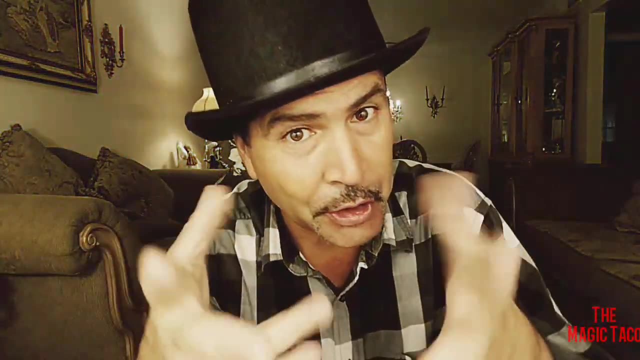 rises up in the air like that. Anyways, I'll tell you the secret right now. Alright, boys and girls, before I show you the secret, I want to let you guys know that every Friday I'm gonna keep posting videos So y'all can learn some more. 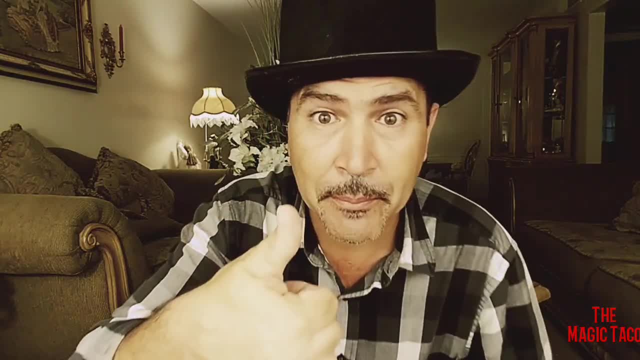 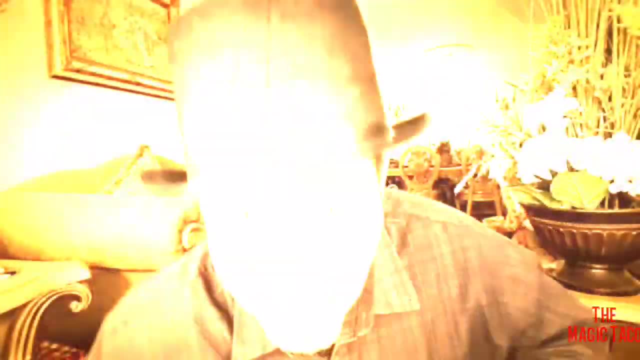 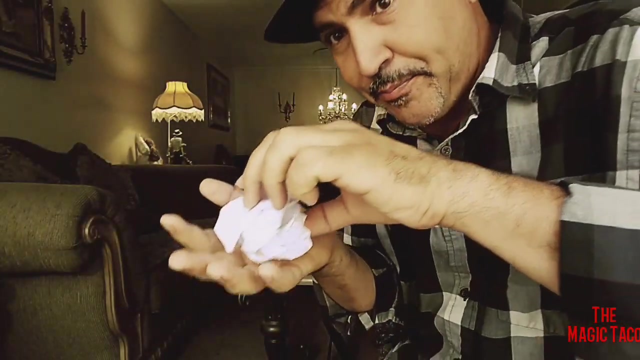 magic. Also, if you like the magic, give it a thumbs up if you don't give it a thumbs down. and don't forget to subscribe. Anyways, check out the secret. and now for the secret. Alright, here's the secret. Place it right here and all. 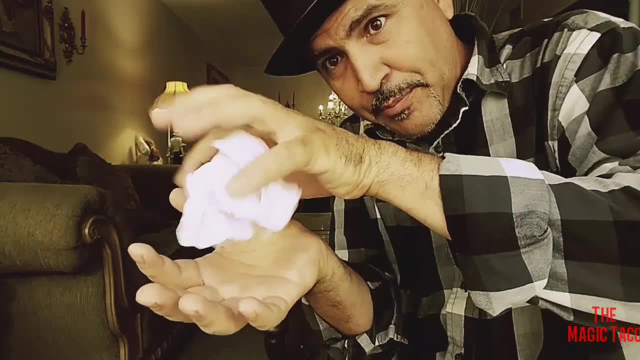 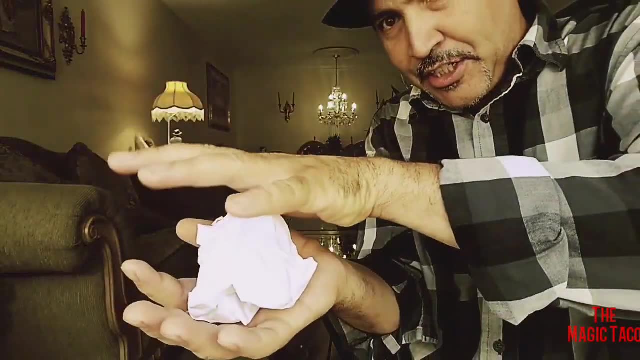 you do is concentrate on it and just like magic, It starts to rise up and you catch it. the secret is really easy: watch. all you do is just grab it, like so, and just by magic it starts to rise. the reason why is because I got a piece of pen stuck in. 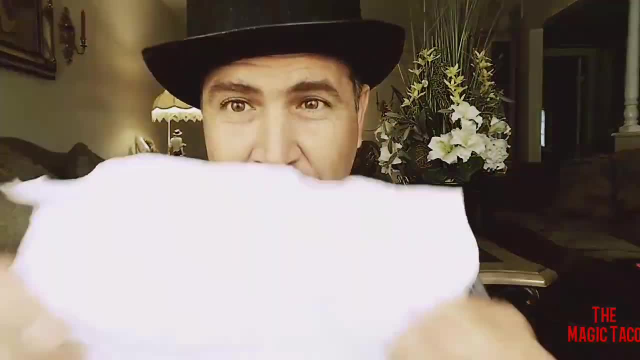 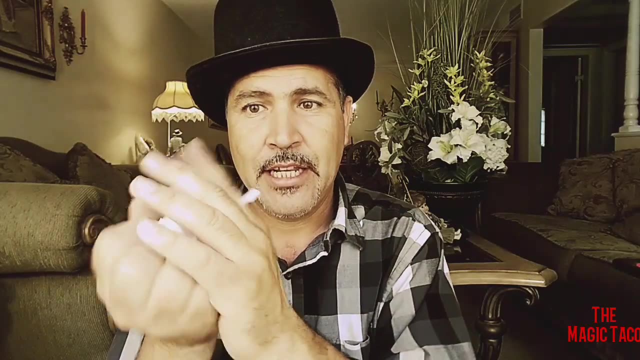 the back. it's a really easy trick and all you do is when you fold the piece of paper, you have the pen behind it, so when you crumble it down, it's gonna crumble on this side and this right here stays sticking out. but of course you. 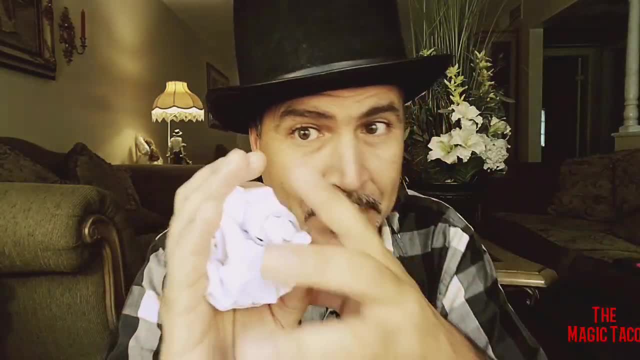 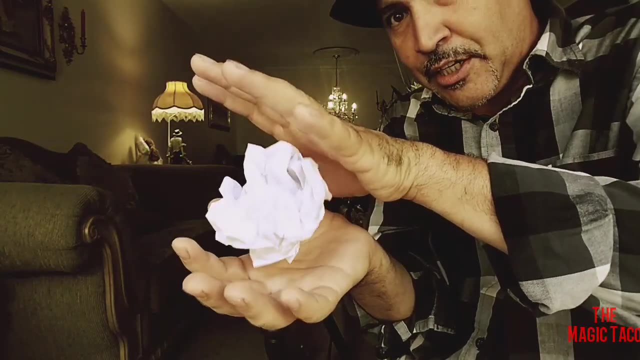 want to have it this way, so they can't see the stick from the front, just like that. you wave your hand and just push behind here. you're gonna push down and it rises up, so push it down and make it look like it floats up in the air. you.